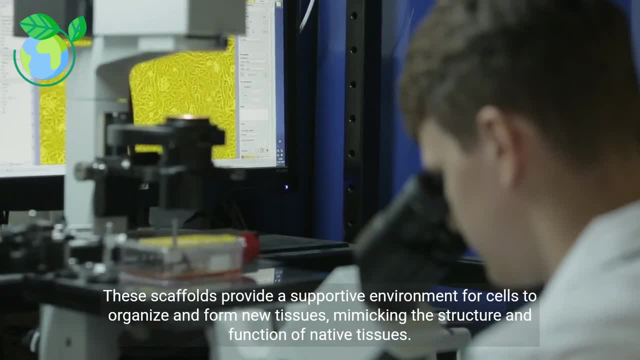 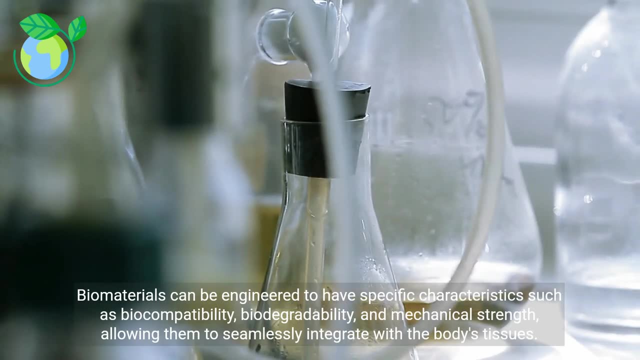 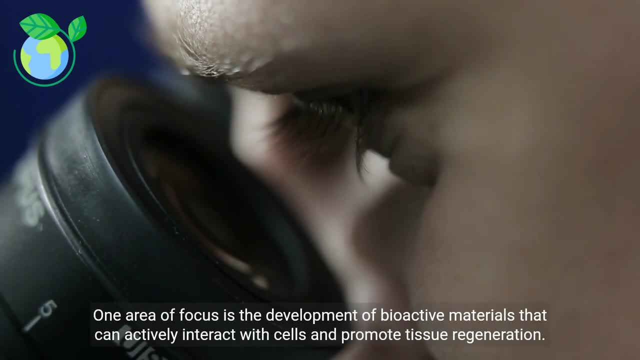 Biomaterials can be engineered to have specific characteristics such as biocompatibility, biocompatibility and biocompatibility. Biomaterials can be engineered to have specific characteristics such as biocompatibility, biocompatibility and biocompatibility. one area of focus is the development of bioactive materials that can actively interact with cells.